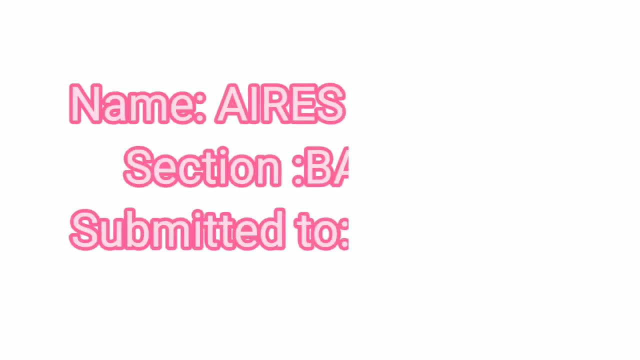 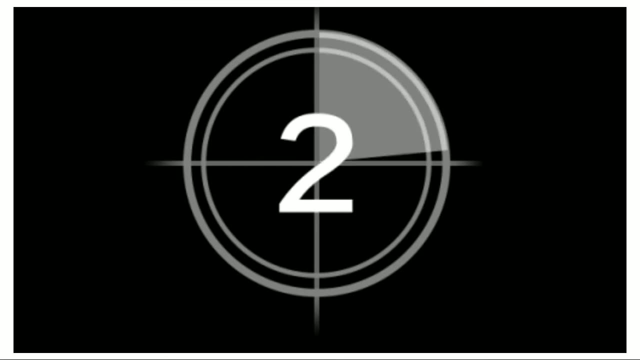 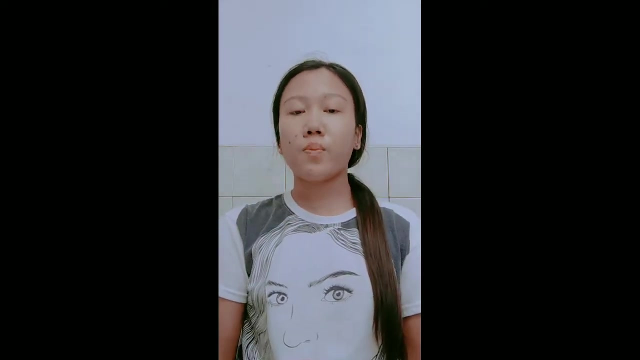 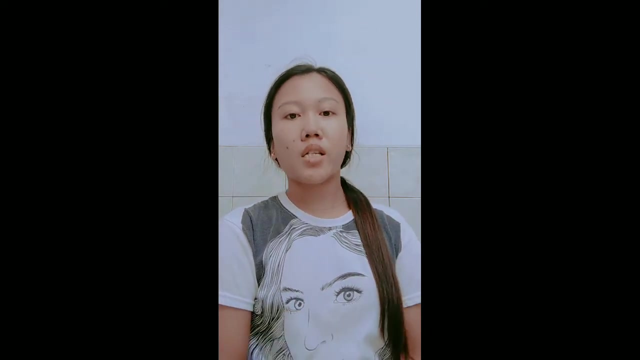 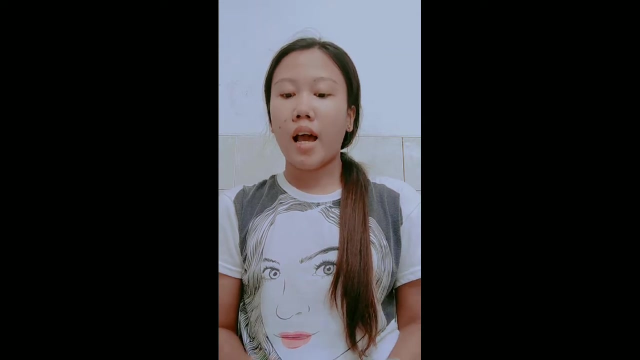 Hi everyone, good day to all of you, especially to our subject teacher, Ms Cha. So for today's videos, I'm going to show you the two practical uses of Pythagorean theorem that can relate to real-life situations. But before with that, I'm going to tell you about 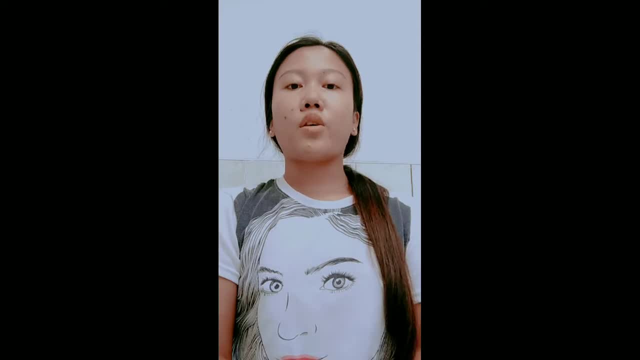 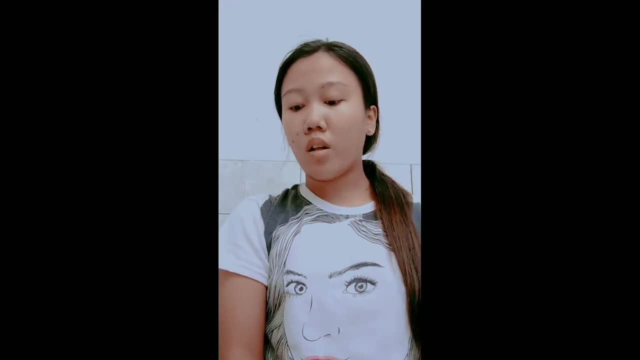 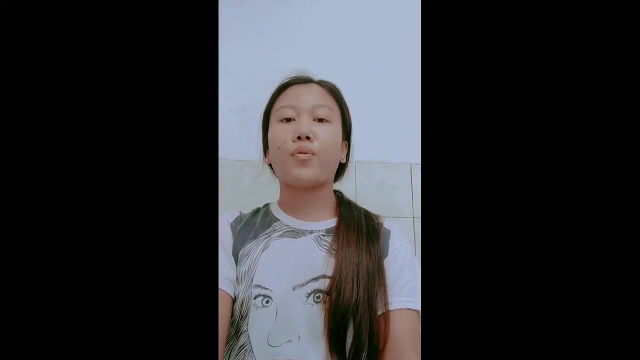 what is Pythagorean theorem? So Pythagorean theorem is a theorem that attributed to Pythagoras that the square of the hypotenuse of a right triangle is equal to the sum of the squares of the other two sides. To know about the Pythagorean theorem, so the formula of Pythagorean. 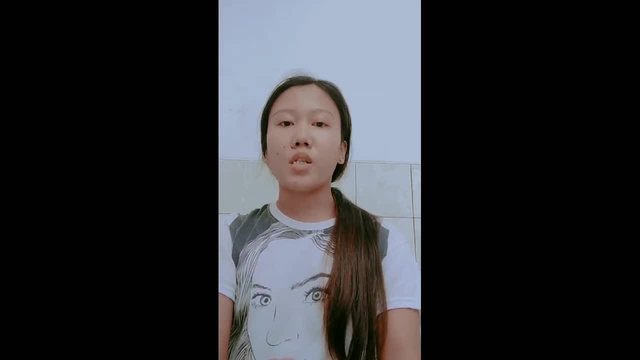 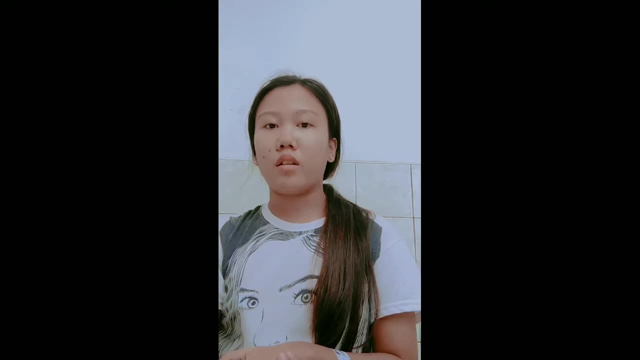 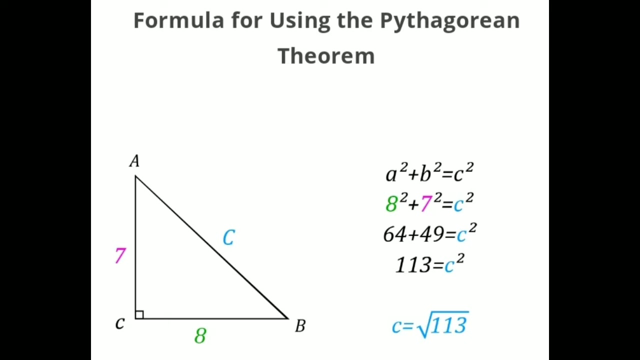 theorem is: a squared plus b squared equals c squared. So a squared plus b squared is the two legs of the right triangle, Then the c squared is the hypotenuse. So this is the formula for using the Pythagorean theorem. So now here are the two practical uses of. 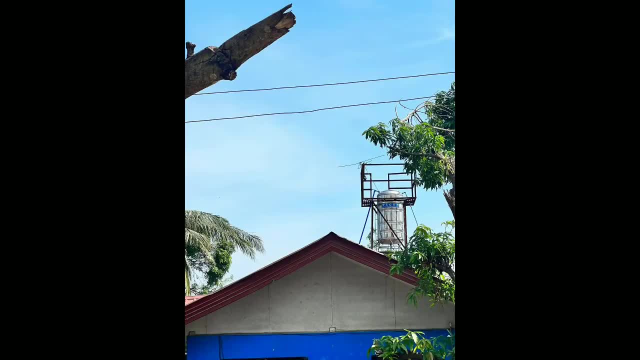 Pythagorean theorem. This picture that I've shown to you now is part of the house, and this can relate to my real-life situations, because this is important to me, because I'm so thankful to the construction worker who built this house, because it is very strong. 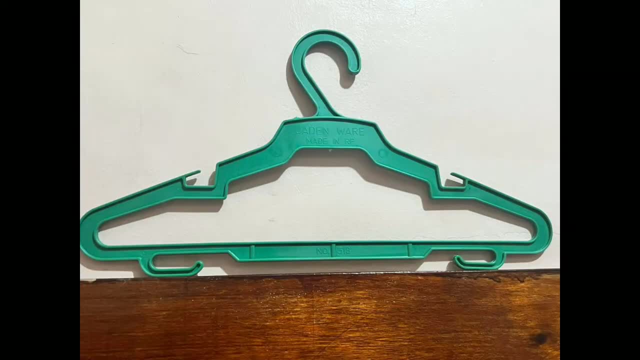 and the measure of its length is perfect. And the second picture is this kind of thing that we've called it hanger. This kind of thing is useful for us and others because it facilitates the hanging of coat, jacket, sweater, shirt and blouse or dress in a manner. 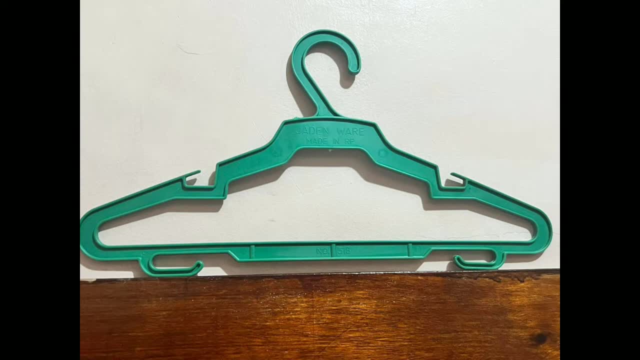 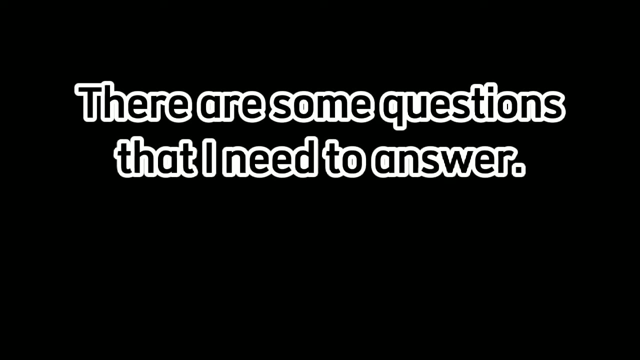 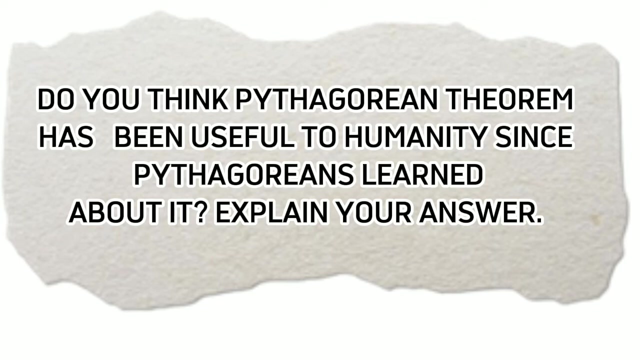 that prevents wrinkles, So it's very useful, And That is why that this can relate in my real life situations. There are some questions that I need to answer, So the first question is: do you think Pythagorean theorem has been useful to humanity Since Pythagoreans learn about it? explain your answer. Yes, of course, because Pythagorean theorem helped us to measure the important things that we do, like we build a house or anything, so it's need a measure so that we will know the exact measure of its size. and it's very useful to our humanity because without 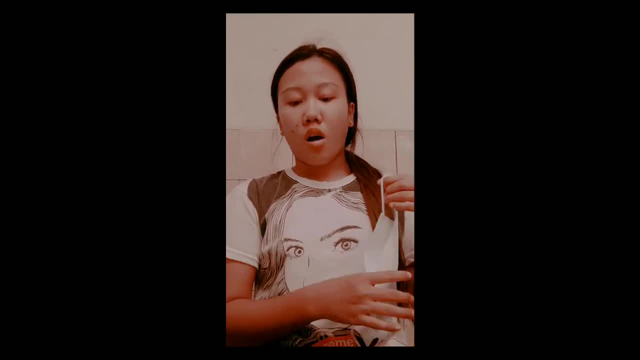 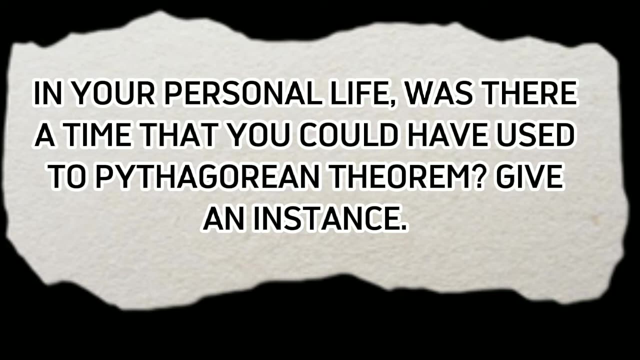 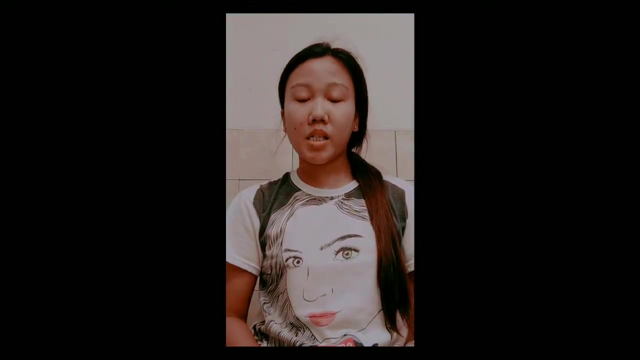 This. we didn't know the measure of the things that we do. The second question: in your personal life, was there a time that you could have used to Pythagorean theorem, given instance? Yes, when I was in elementary and high school, I used one paper and pencil.